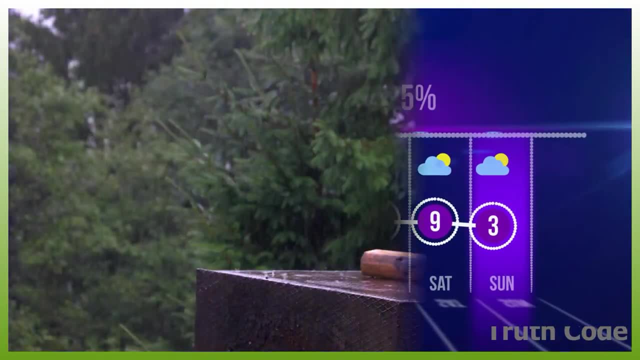 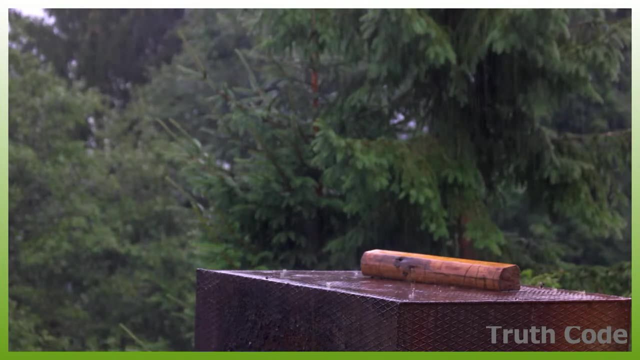 probably just checked the weather forecast. Weather forecasts help us prepare for the future, whether it's a few hours from now or the rest of the week. Not only do they warn us of potentially dangerous weather headed our way, they also give us an idea of what. 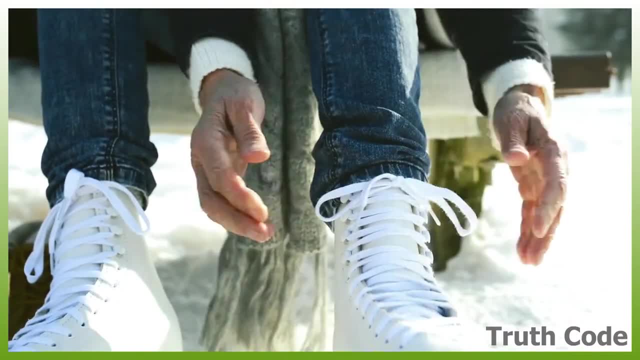 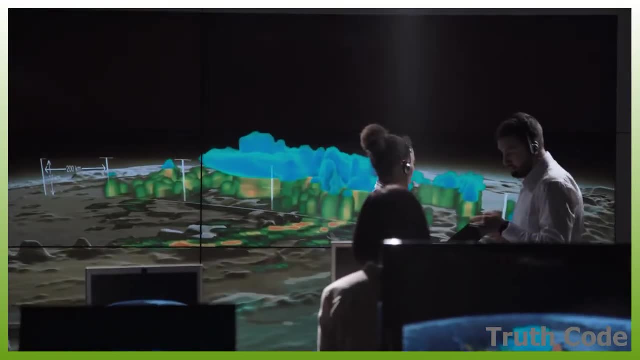 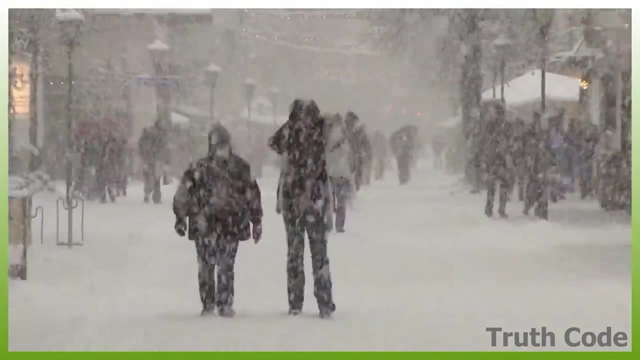 to expect in terms of temperature and chance of precipitation, so we can dress and equip ourselves appropriately. The people who study the weather and put together forecasts are scientists, known as meteorologists. Have you ever seen a forecast that called for lots of snow? You might have gotten excited, anticipating a snowy day and the chance to do some sledding. 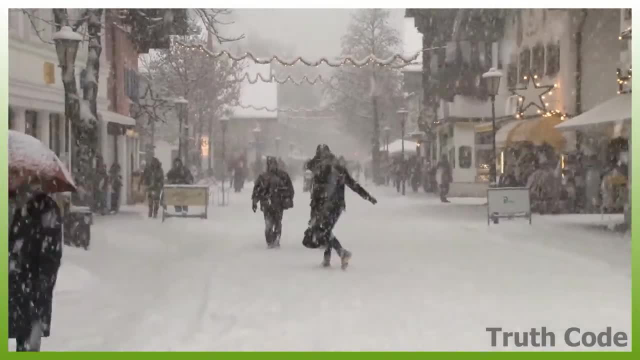 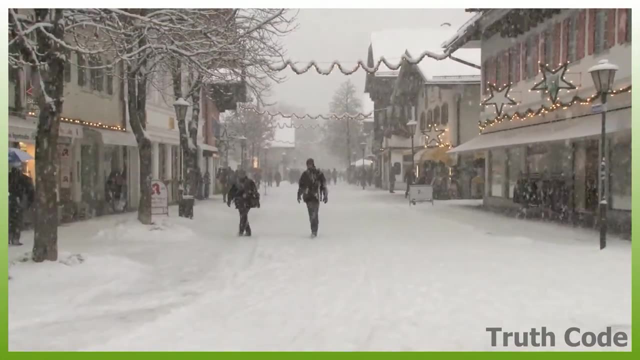 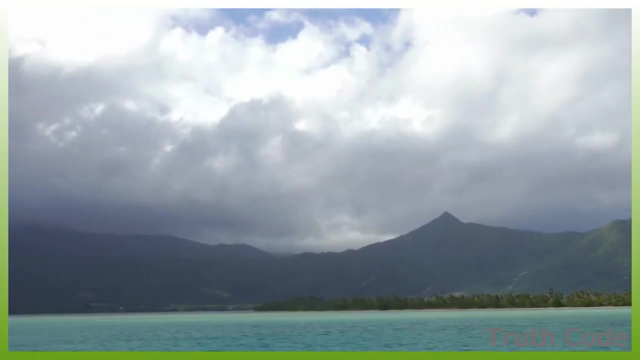 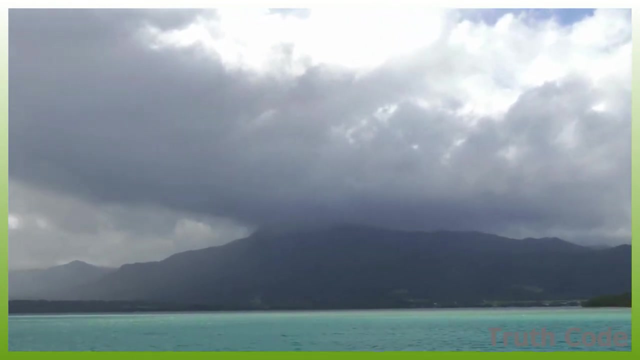 but unfortunately you woke up to clear skies, no snow and a full day of school ahead. What happened? Could the weather forecast have been so wrong? Weather forecasting is not a perfect science. Forecasts are a prediction based upon an educated guess. Since there are a wide variety of factors that go into a forecast, it's possible for 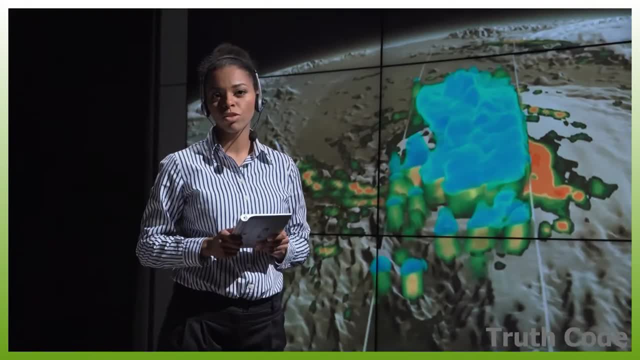 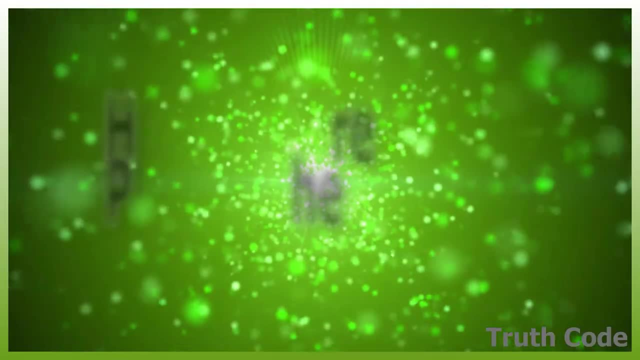 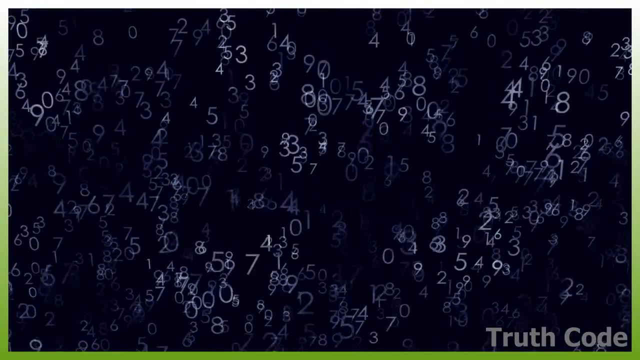 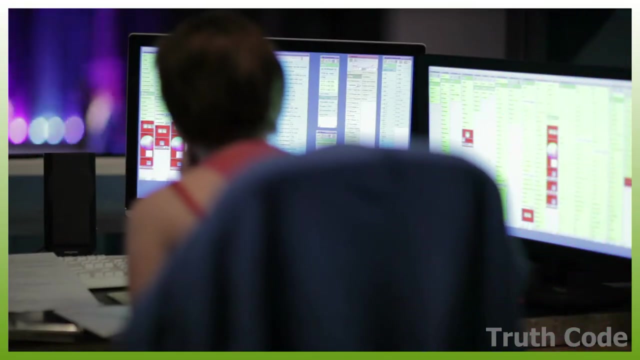 meteorologists to guess wrong from time to time. Fortunately, modern technology has allowed forecasters to become much more accurate over the last decade. Today, meteorologists use complicated mathematical equations to help predict the weather as part of a process known as numerical forecasting. Numerical forecasting requires powerful supercomputers. 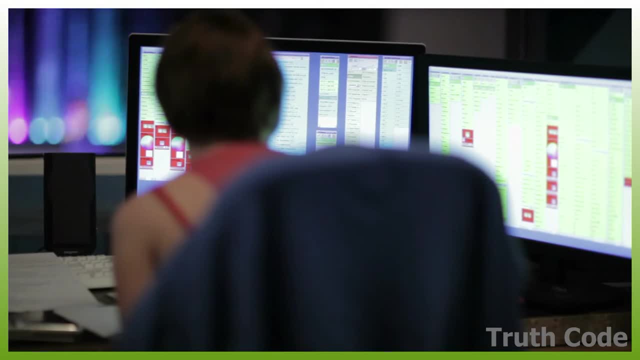 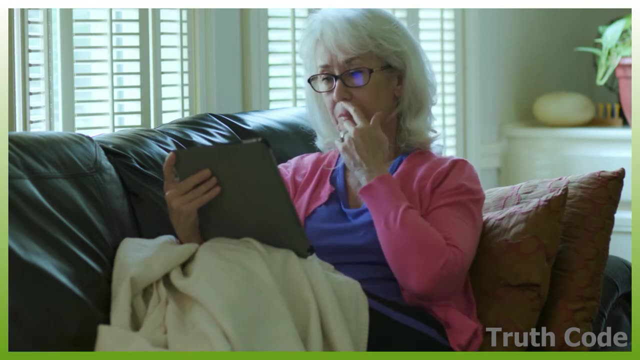 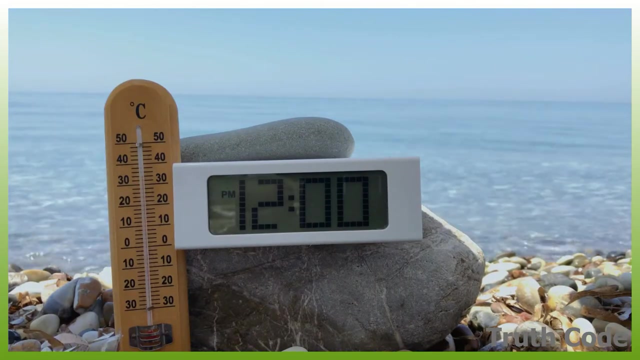 and tons of observational data from land, sea and air weather stations around the world. But where does all this data come from? Sometimes it comes from regular people like you. Many people create their own backyard weather stations with thermometers to measure temperature and precipitation. They can report their observations to local meteorologists to help improve local 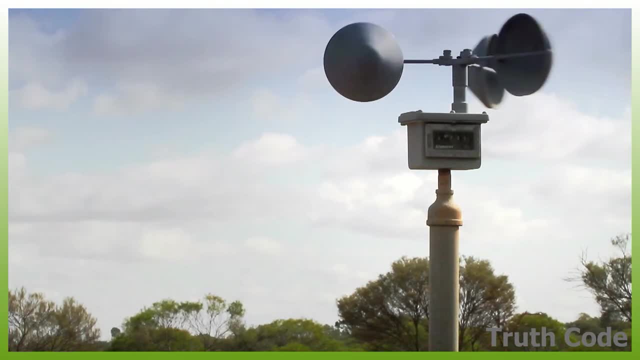 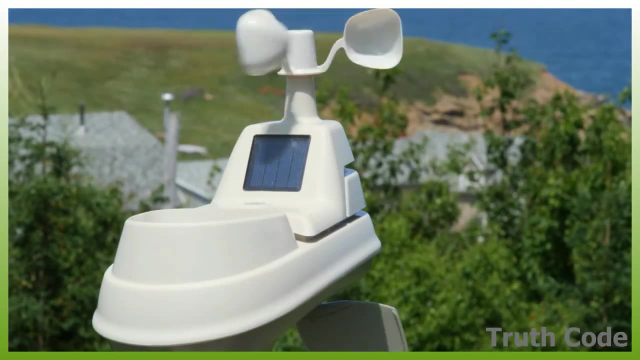 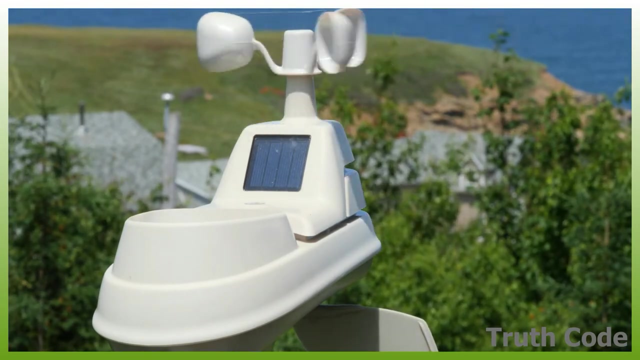 forecasts. Technologically advanced weather stations are established by meteorologists all over the world. They collect and share data to help improve forecasts. Some of the tools they use include barometers that measure air pressure, anemometers that measure wind speed, Doppler radar stations to monitor the movement of weather fronts, and psychrometers.